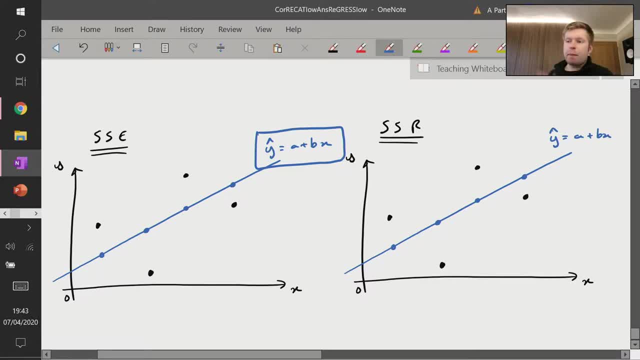 is y hat. so that's the estimator is a plus bx. the way in which we defined the values of a and b was simply by thinking about the distances between where our actual data value lies and where our estimated data value lies, And we called those values residuals And 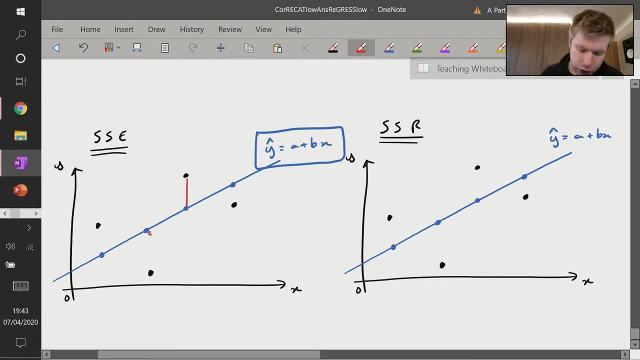 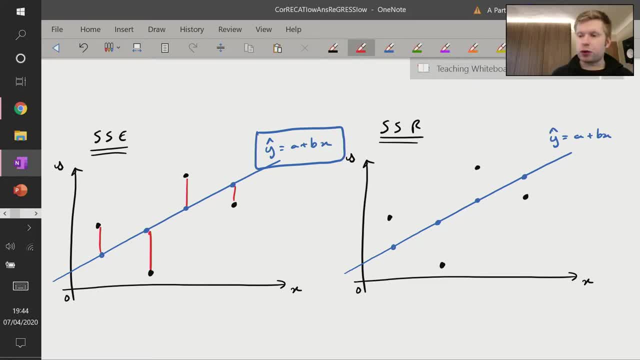 OK, Now, the name which we gave to that was the least squares regression line right, and that's literally how we came up with the regression, And we can quantify the error in three different ways. OK, so if we want a really, really good regression line, we 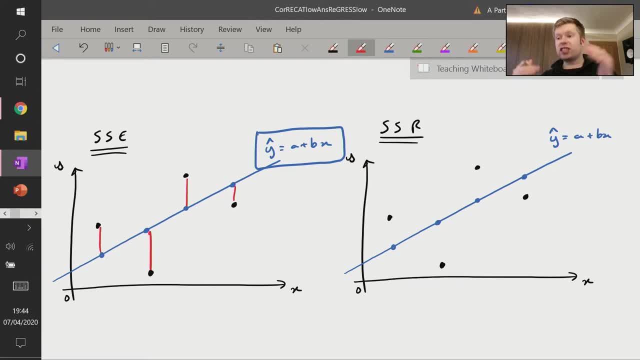 should look at these three different quantities and then we can quantify them and sort of see actually how good is our regression line. So the first way that we've already looked at is the idea of the sum of the squares. error. OK, so this stands for the sum of the squares. 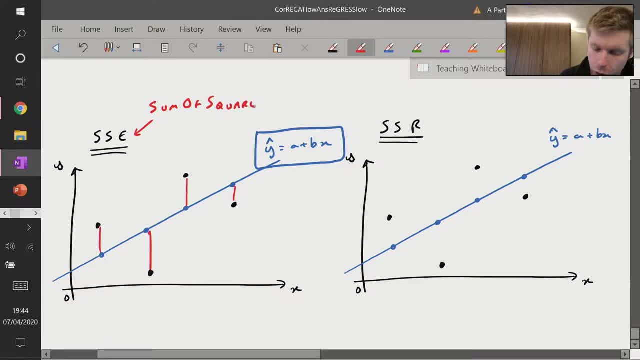 The sum of the squares error, Or we can call that SSE for short. OK, so the sum of the squares error. It simply looks at the differences between our actual data values. so these are our actual data values, so like y1, y2, y3, so y1, y2, y3, y4, and our estimated data. 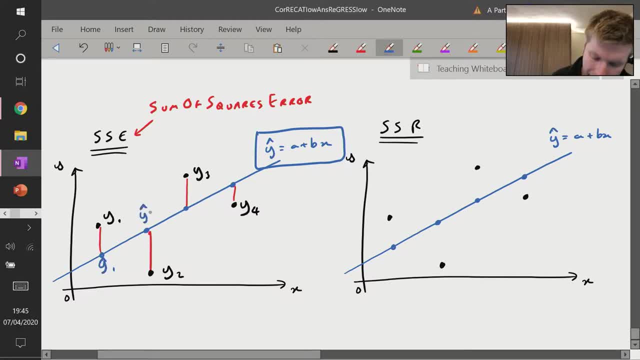 values. OK, so this would be like y hat 1 and y hat 2 and y hat 3, et cetera, Because we're actually basically saying that when we draw our regression line through these points, we're basically saying that the trend of the data follows this regression line. 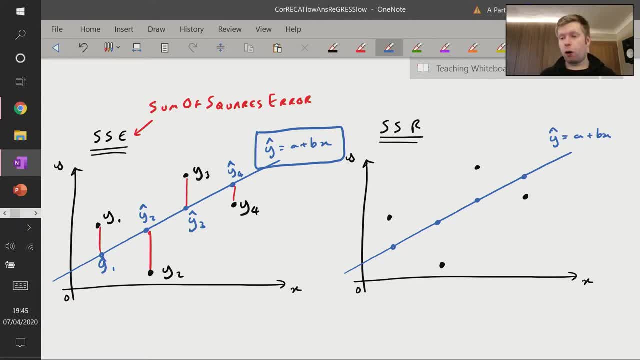 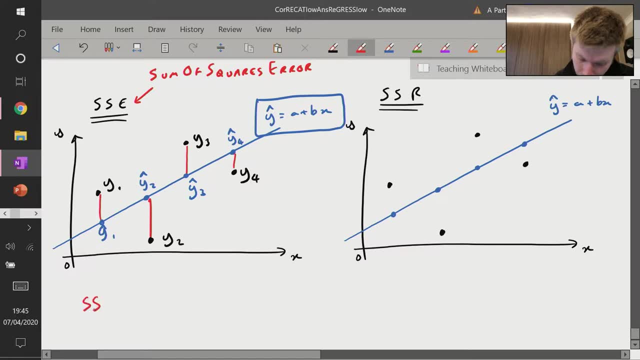 And so, therefore, if we want to estimate these values, they should lie on the regression line, So, in other words, a way of quantifying the sum of the squares error. the sum of the squares error is simply, by saying it's the difference between our actual data values. 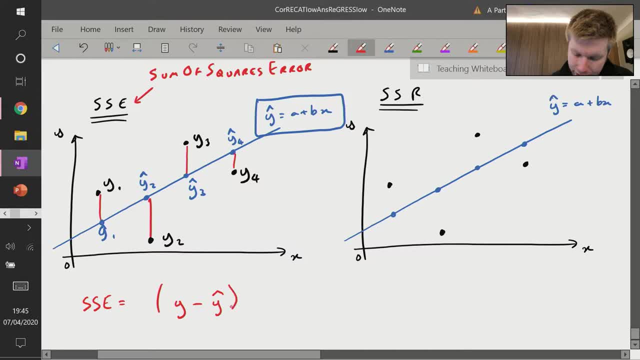 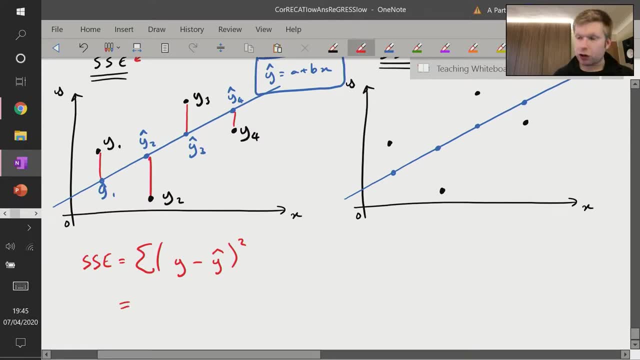 take away. take away our estimated data values, square that And that's it And then add it. OK. so we've already met this formula before And in fact we said: because each of those lines are really important, so the little red lines are important. we 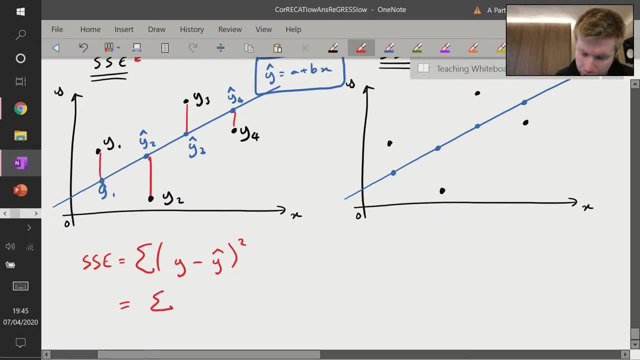 call those residuals. it's simply just the sum of our residual squared. OK, so, sum of our residual squared. All right Now. in actual fact, we came up with a formula for the sum of the residual squared. We called it the deviance or we called it the residual sum. 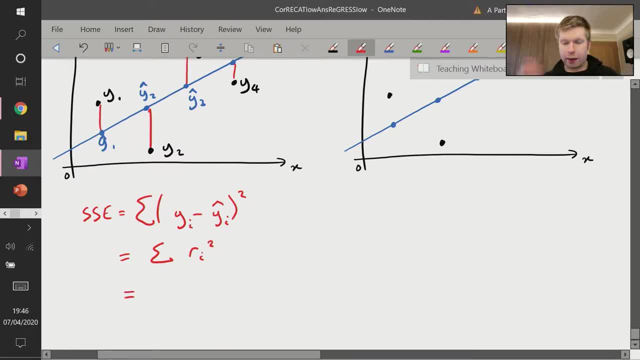 of squares. OK, and if you remember, it was a weird formula which came out in the last video, So we did this. It was SYY minus SXY, all squared divided by SXX. OK, so once we'd found the 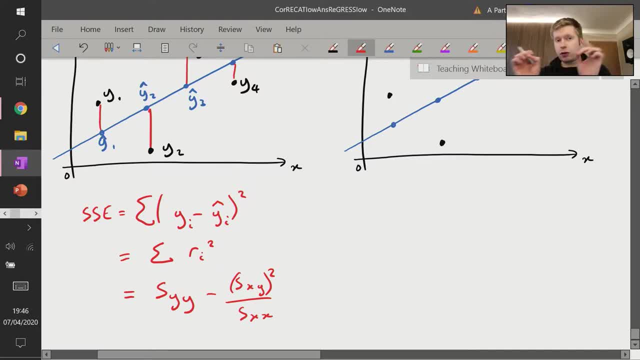 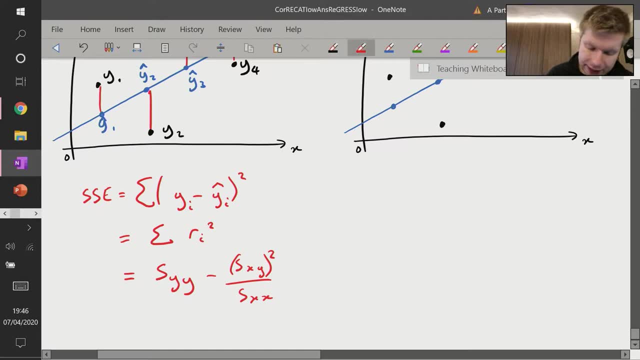 values of A and B, we realized that choosing careful values of A and B could make terms completely disappear, And what we would have been left with is this: OK, so what we can basically say is that the sum of the squares error can be given as this: 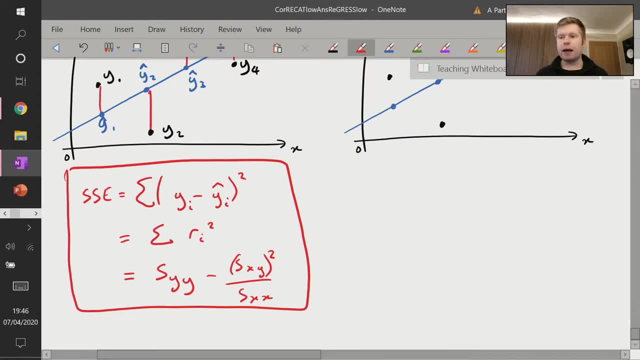 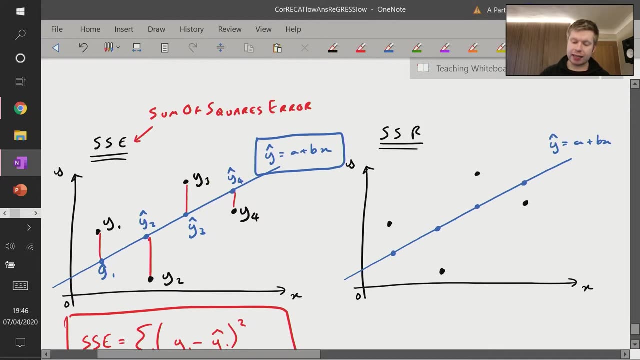 And the idea is that choosing the correct values of A and B should make this as small as we possibly can. So we quantified the error in one way, OK, But my question is: are there any other ways that we could quantify this error? And the answer is yes. 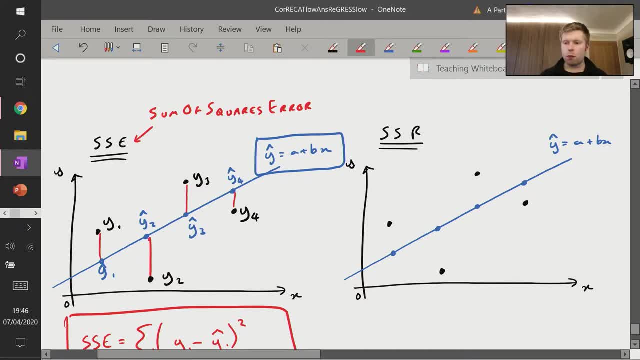 So let's suppose we came up with the regression line, OK, And at the moment we're looking at the difference between our actual data values and our estimated data values, in other words, where the regression line says those data values would lie if the data properly. 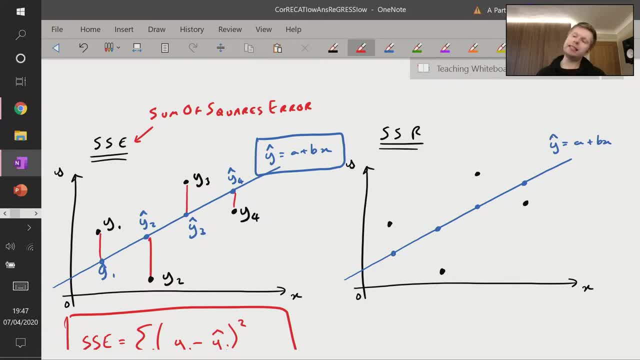 followed that regression. OK, And so is there any other way that we can quantify this? Well, the answer is yes, And the way to do this is by looking over here on the right-hand side. So, looking at this plot here, Now what I'm. 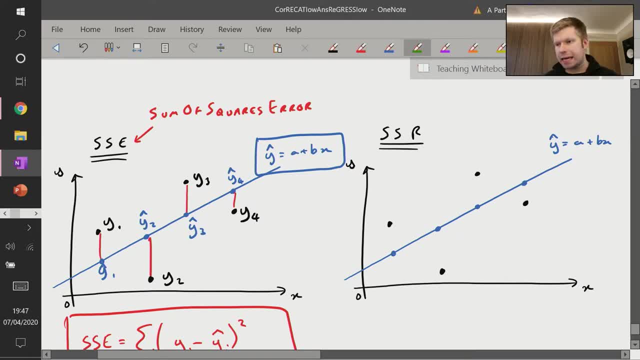 going to do, first of all, is I'm going to calculate the mean of the data values which I've got. So if this is again so, for example, y1, y2, y3, these are my dependent variables. okay, I'm simply going. 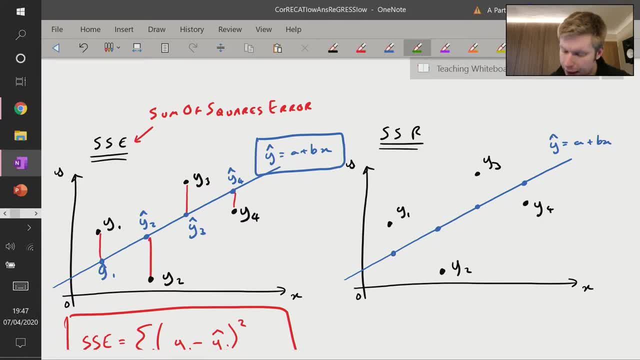 to take the mean of those dependent variables and draw them on. So let's say that the mean ends up somewhere about there. okay, In fact it might be a bit higher, It might be, I don't know about there. say okay, So I'm going to call that y bar. okay, That is the mean of my y values. 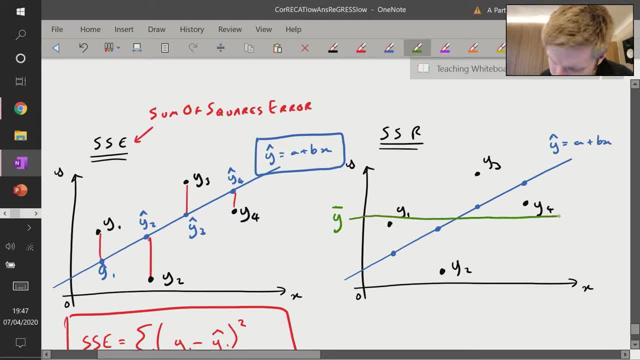 okay, The mean of my dependent variables. okay, And what I'm going to do then? what I'm going to do is look at the difference between where my estimated values are, So that'd be y hat 1, y hat 2, y hat 3, etc. I'm going to look at the difference between the. 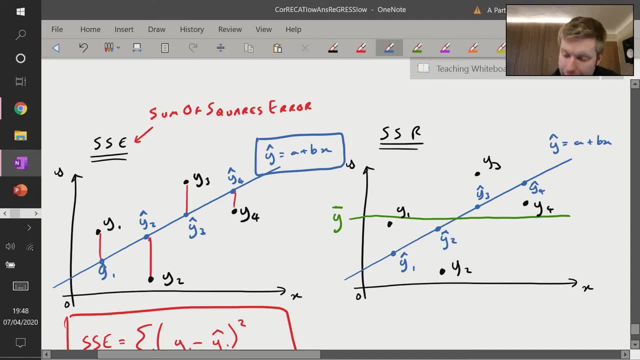 estimated values okay, and where the values actually lie. So, in other words, I'm going to look at this distance here. So I'm going to look at the distance between my estimated value and the mean value And that's what I'm going to call the sum of the squares- regression, because I'm 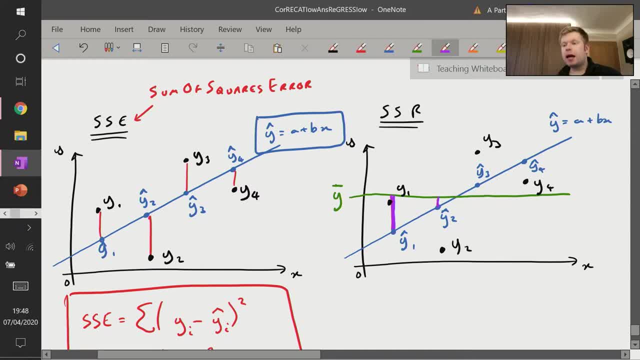 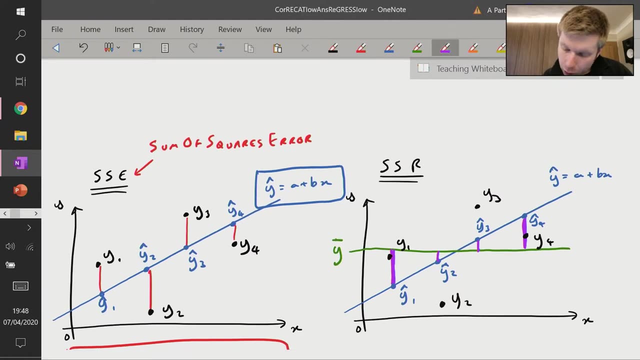 simply looking at the difference between my regression values and the mean value. Okay, so I'm trying to quantify the regression values by looking at the difference between the estimated or the regression values and the mean value. So in other words, I can say the SSR which I'm 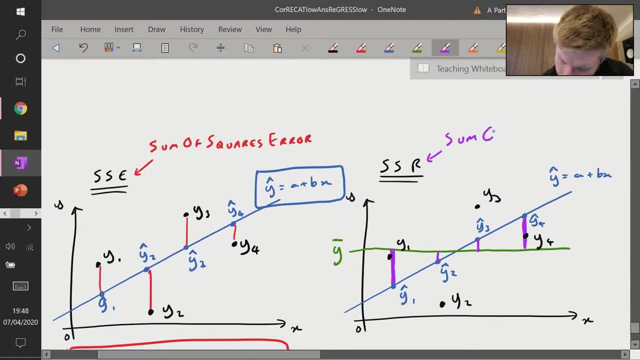 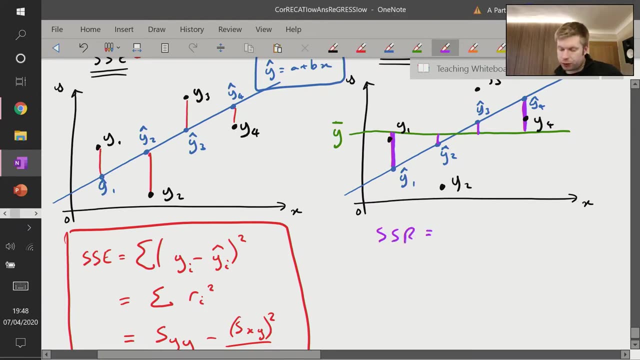 calling the sum of the squares. regression is given by looking at the difference between- obviously I'm going to do the square difference because I want them all to be positive- okay, Between my estimated value, so y bar and my sorry y hat and y bar my mean value, okay. 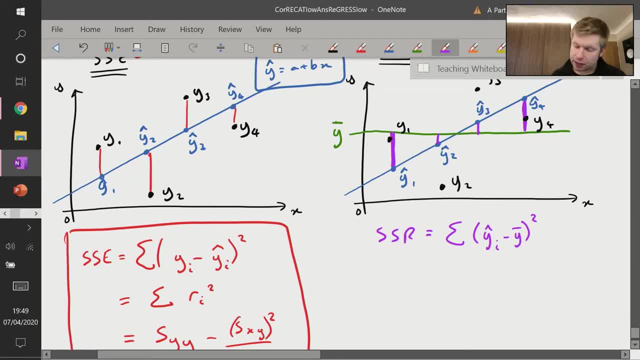 so y bar okay. Now, in actual fact, I'm going to come back to this formula a little bit, because we can actually use it in terms of SXX and SSY, et cetera, et cetera. So the next thing to look at: 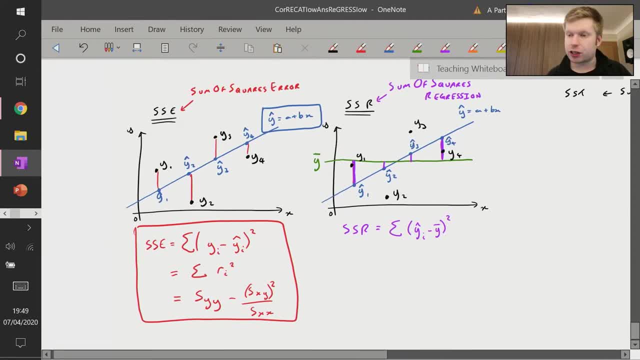 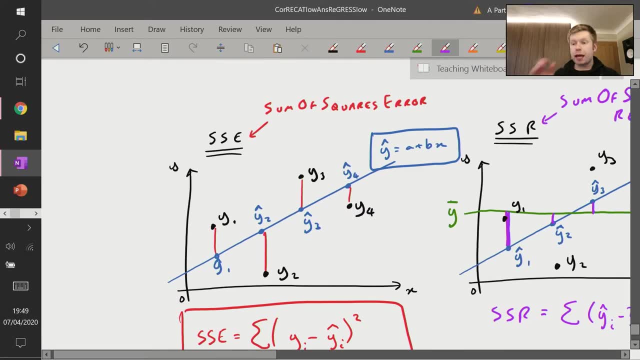 is something called the total of these two errors here. So I've got the sum of the squares error and the sum of the squares regression. Now, what I want to do then is I can combine these together to make it to kind of quantify the total error, if you like. okay. So the last thing I'm going to 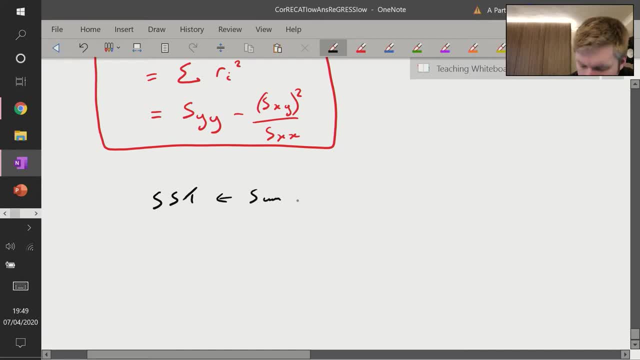 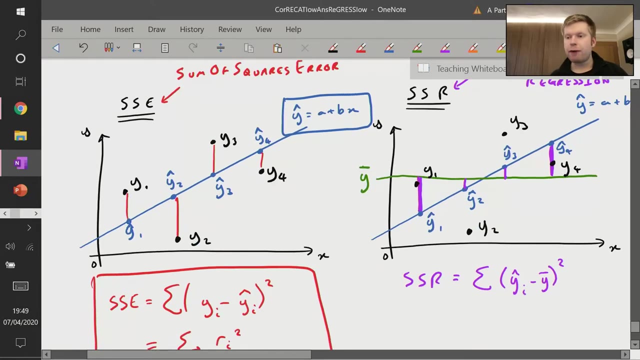 look at is the SST, which is the sum of squares total, And all it literally is is: you're literally taking the two previous errors that we've looked at. so the sum of the squares error- that's this one here on the left, okay- is literally looking at the difference between the actual data value. 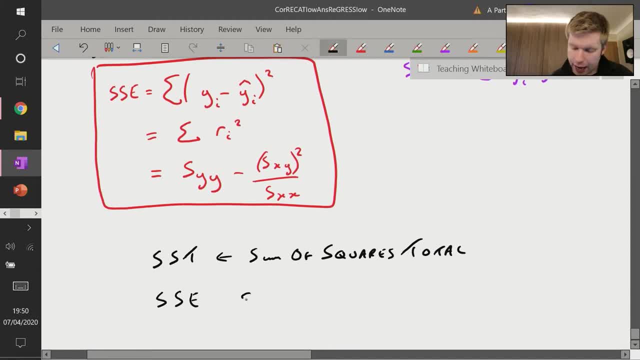 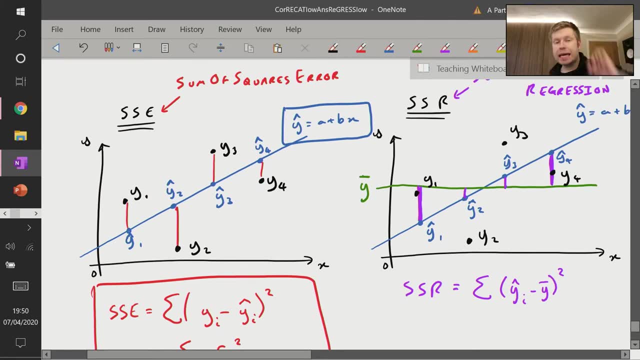 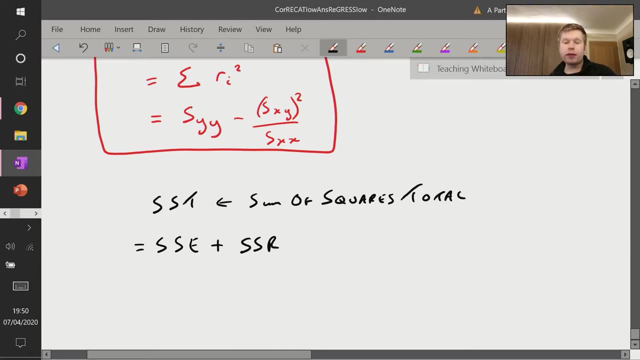 and the estimated data value. So I'm going to look at SSR, which is the sum of the squares regression, which is simply the difference between the regression values and the mean of my data values. okay, and then I'm just simply adding them together. So the sum of the squares total should be the total of these two. 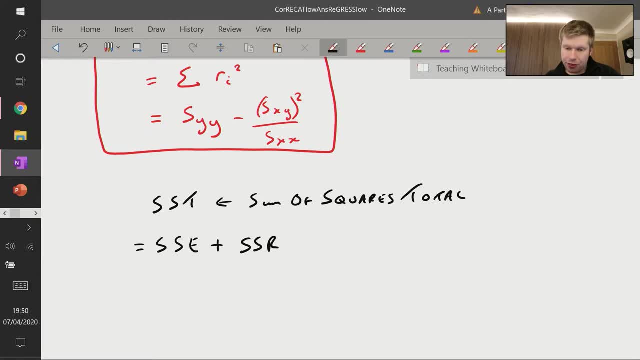 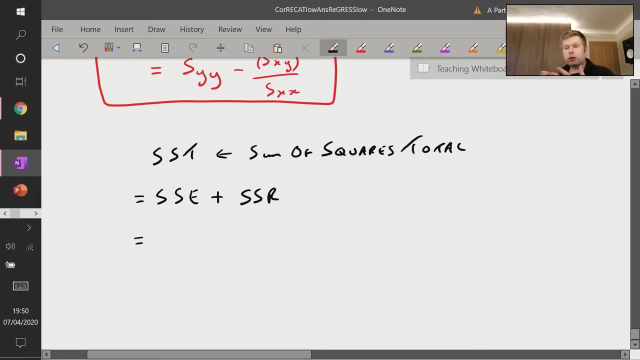 errors here. okay, Now have a think about this. have a think about this. I've literally said that the sum of the squares total should be the total of the two errors. So, in actual fact, I'm just going to draw out on a new grid. I'm just going to draw out on a new grid. I'm just going to draw out on a new grid. 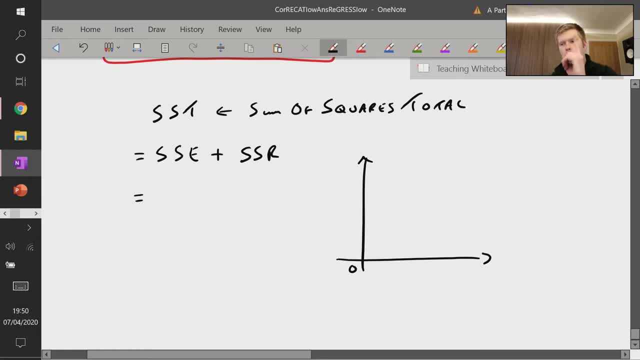 what I've got here. So I'm just going to draw it out for one data value. So let's suppose that I have my true data value all the way up here, so this could be like Y1, okay, Then I have my regression, so my 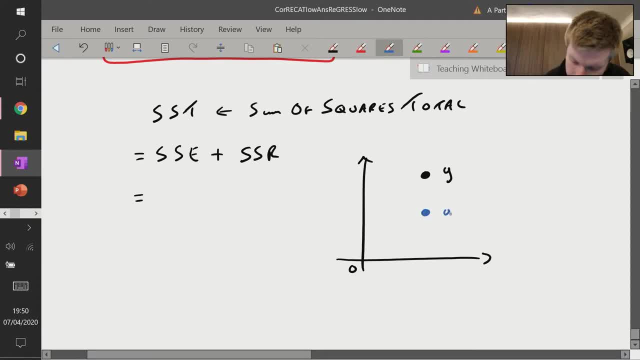 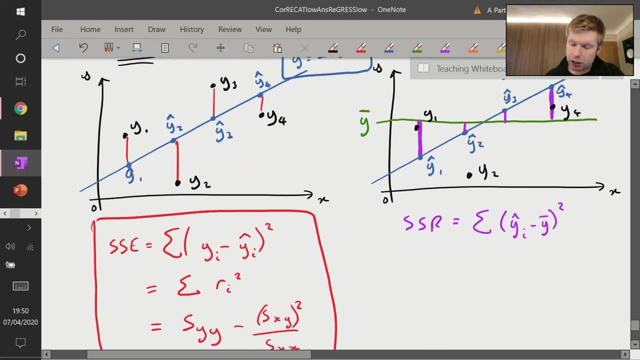 estimated data value here. okay, so I'm going to call that Y hat And then let's suppose that the mean of my data value lies down here. So what I'm literally looking at here is kind of on this graph, on the right hand side graph in fact, just because it's a little bit messy, have a look at the screen. 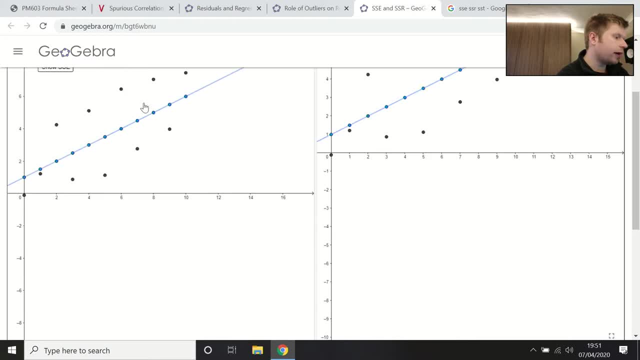 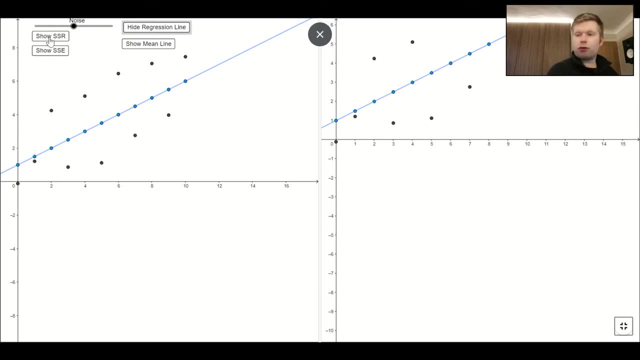 here. okay, So I've got sum of squares. I draw my regression line. okay, draw my regression line. let's make that full screen. got my regression line there. Some of the squares, some of the squares. error is going to be the difference between my actual data values in black and my 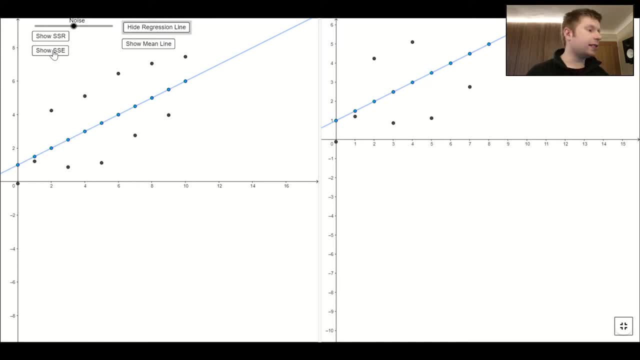 regression data values in blue, in other words the values that lie on the data on the regression line. So that's in red there And some of the squares. regression is simply. if I was going to draw in the mean line, which I've done there in green on the right hand side, let me get me. 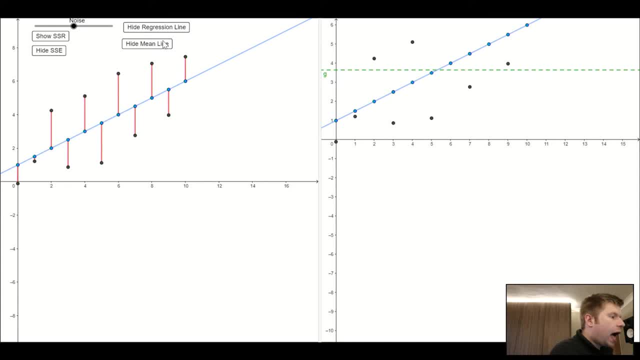 out of the way, okay, which I've done there on the right hand side, And if I was going to look at the difference between where the mean value is and where the regression value is, that there would be the sum of the squares regression, okay. So all I'm literally trying to do then, all I'm literally 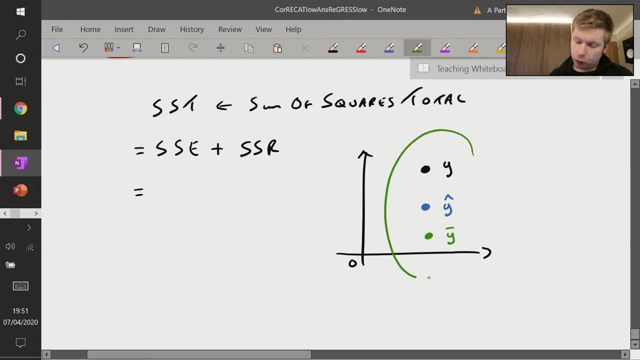 trying to do, then, is try and quantify it Now. of course, it could fall in this order, so I could have the actual data value at the top, then the estimated data value in the middle and then the mean data value at the bottom, or I could have it in any kind of permutation of these three things. 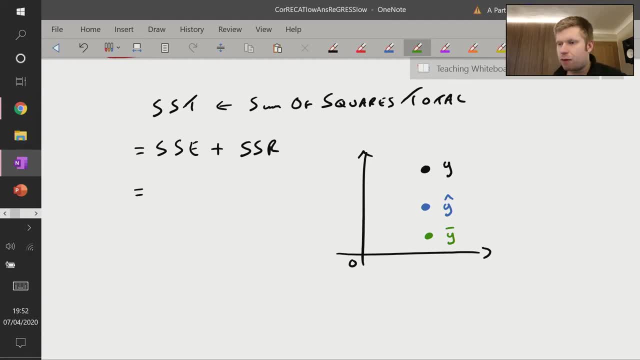 And, of course, they're always going to be in line, because I'm looking at that in relation to the independent variable. So what I've looked at, then, what I've looked at just to remind yourselves the difference, the difference between y, hat and y. so my actual data value and my estimated data. 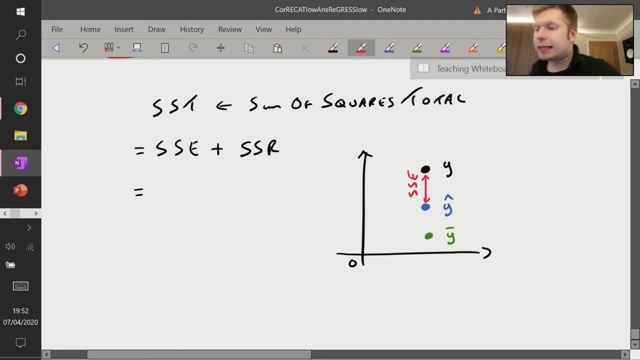 value I have called the sum of the squares. error, It's literally just my regression, okay, So I've looked at the squares of those distances and summed them all together. Now I've looked at the difference as well between my estimated data value. so, in other words, my regression data value. 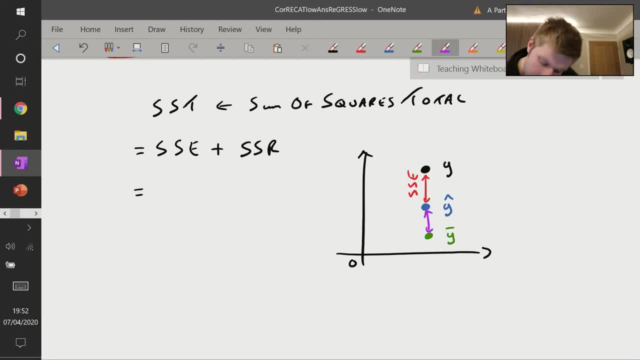 and my mean data value, and I've called that the sum of the squares- regression. okay, So it's SSR. right Now, I'm literally saying that the total of these two errors is going to give me guess what? the sum of the squares total. the sum of the squares total. okay. So let's think about this. 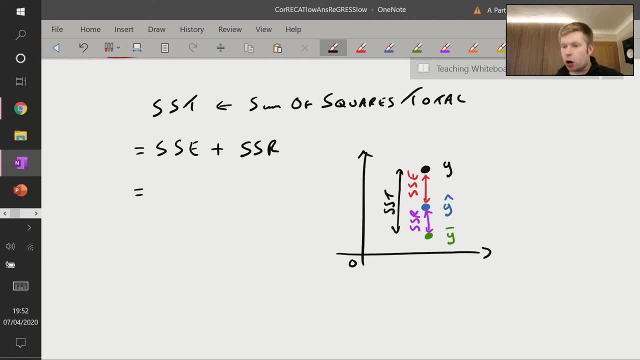 let's think about this right. Some of the squares total I can think about as the total distance between the extremes. In other words, I can think about it as the sum between y and y bar all squared, Because, look at that, it is the distance between. 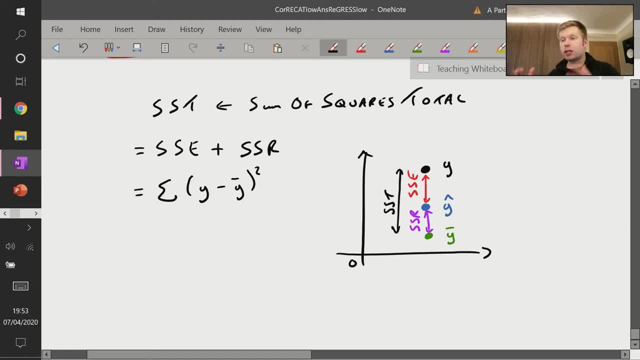 y and y bar. Now, the fact that these can come in any order doesn't matter, because the maths actually falls out, but I'm going to square that Now. have a look. I recognise what that should be equal to. I've seen a formula like this before. It's just SYY, okay. So in other words, I can say: 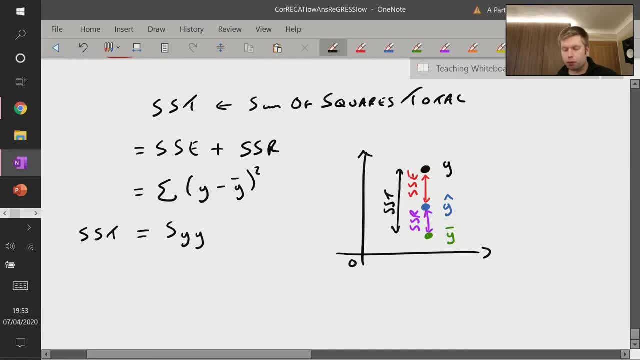 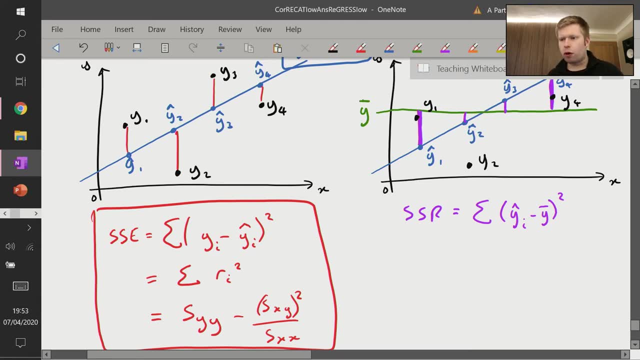 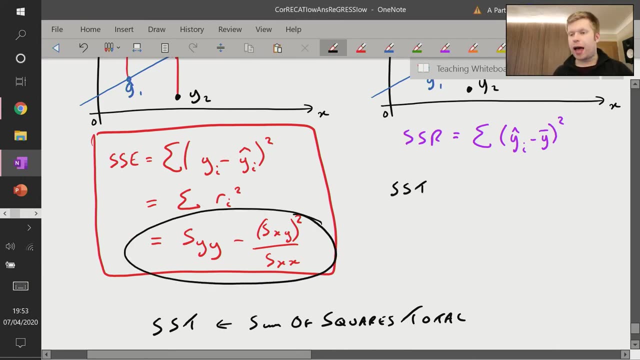 SST is equal to SSY. So let's just remember when I came up here and I said: oh look, SSR, sum of the squares, regression, is equal to. this Looks quite messy and horrible, but if I do just a little bit of rearranging, because I know now what SSE is equal to in terms of SXX, SYY, SXY, 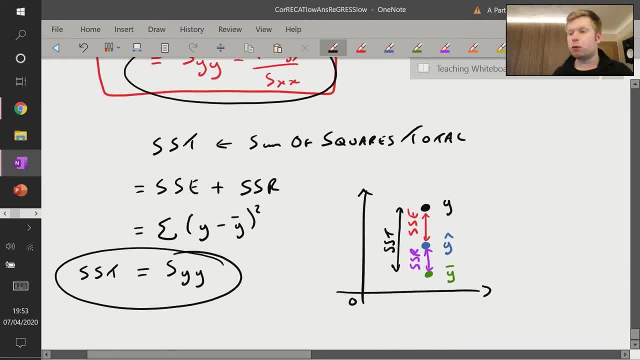 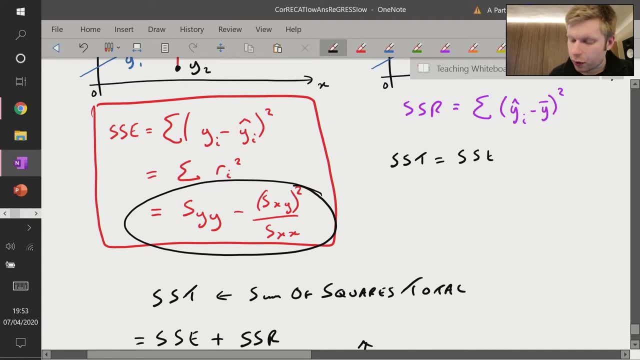 okay, and I know what sum of the squares total is equal to in terms of SYY. okay then I know, after a bit of rearranging, that sum of the squares regression should just be equal to sum of the squares total. take away sum of the squares error. So have a look then. sum of the squares total. 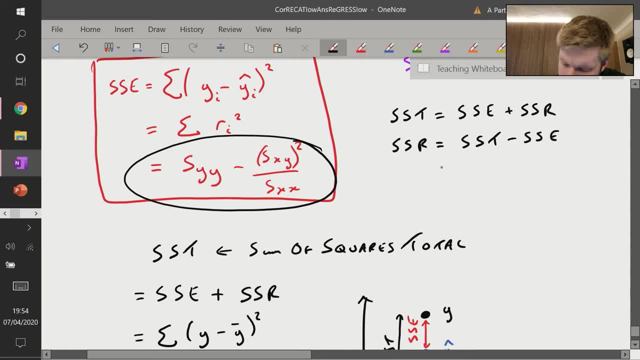 I've said way down here is equal to SYY. So this is equal to SYY. Then I'm taking away sum of the squares error. Well, the sum of the squares error. I've got over here right, So it's going to be. 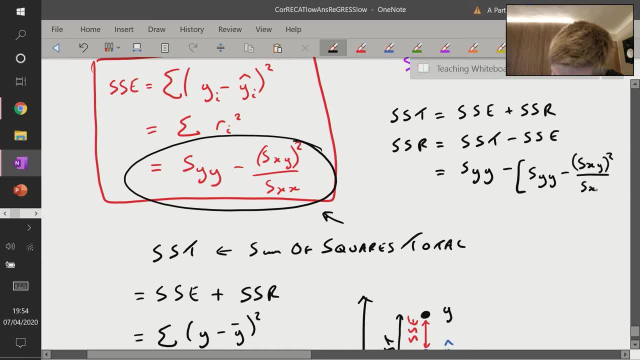 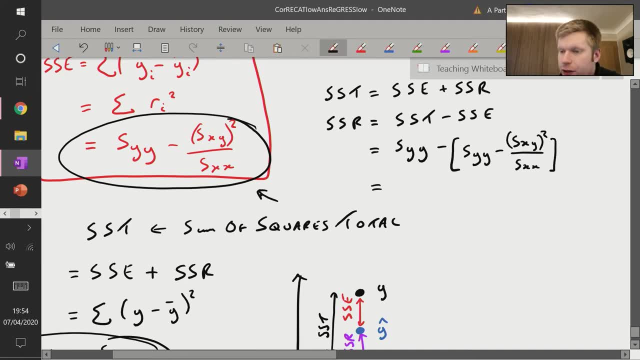 SXY all squared, divided by SXX. all right. So therefore, if I take away these two things from each other, just got to be careful of the double negatives here. In fact, let me make a little bit more space, so I've got room. Just got to be careful of the double negatives. here I end up. 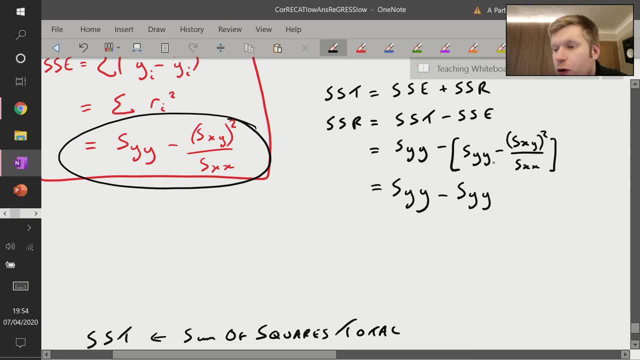 with SYY. take away SYY. Now I've got double negative. taking away a negative is the same as adding a positive. So SXY all squared, all divided by SXX, And of course these two things are equal to SXY. So I've got SXY all squared, all divided by SXX, And of course, 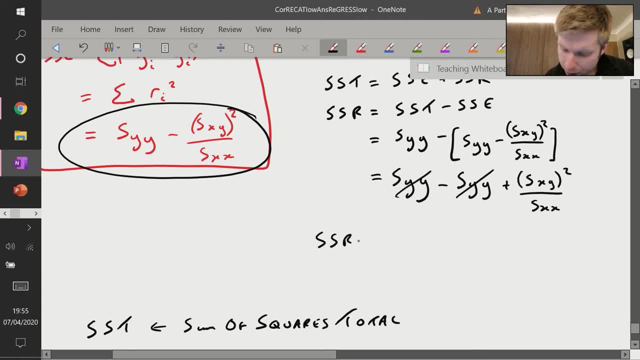 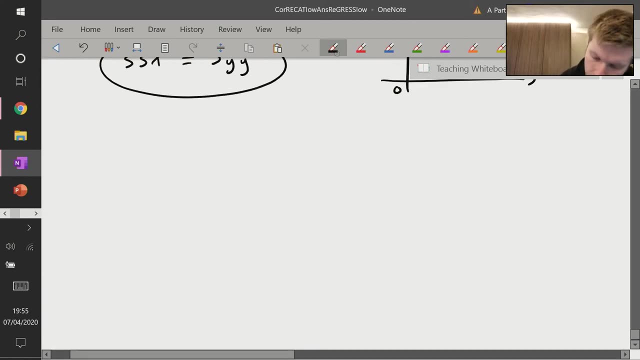 these two things cancel. So in other words I can say that SSR. so my sum of my squares regression line should be equal to SXY, all squared divided by SXX. okay, So just let me summarize down the bottom here. I've got two, maybe three types of errors, depending on how. 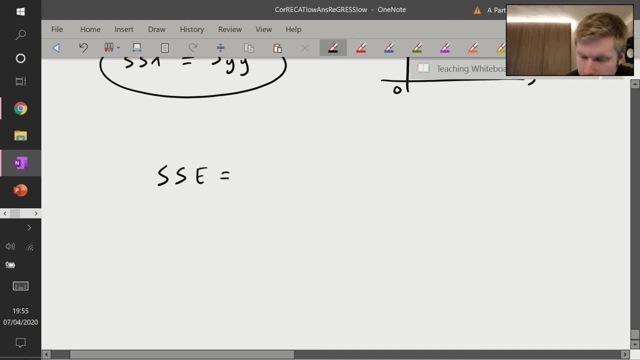 you think about it, We've already looked at sum of the squares. error, That's just equal to the deviance or the residual sum of the squares which, if you remember, was SYY all divided by SXX. Okay, So we divide, we derive that when we're doing, when we're deriving A and B, Okay, We've. 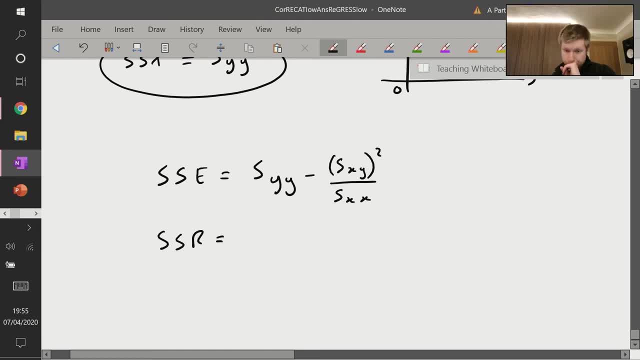 said as well, there's another type of error that we can look at, which is simply just the distance between the regression point and the mean point. Okay, So that's going to be. we've just worked it out as SXY all squared divided by SXX. Okay, And the final error. 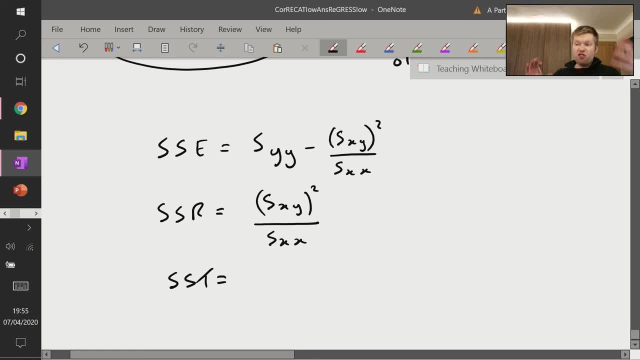 is just simply the total of these two things. Okay, So really, what you want is that these errors are going to be as small as you possibly can, because it means that your data values are going to fit the line quite nicely. And we've just said: 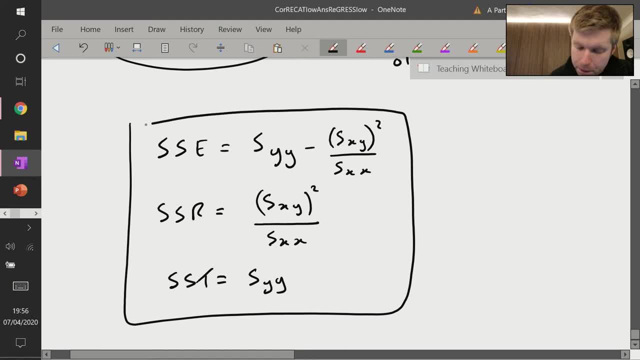 that the sum of the squares total is just SYY. Now just remember, these are really easy to calculate because you know what SXX, SYY and SYY is equal to. So I'll write down the simpler version of the formula which I remember, but of course there are two versions. So SXX is equal.